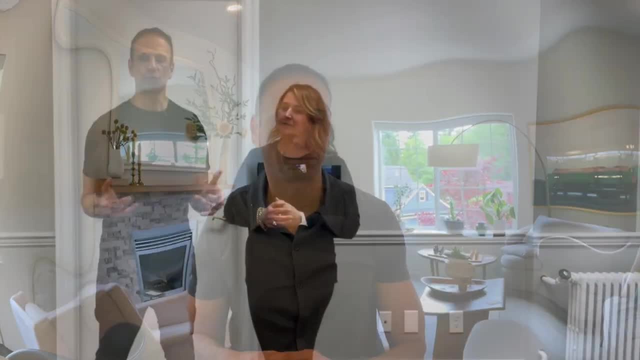 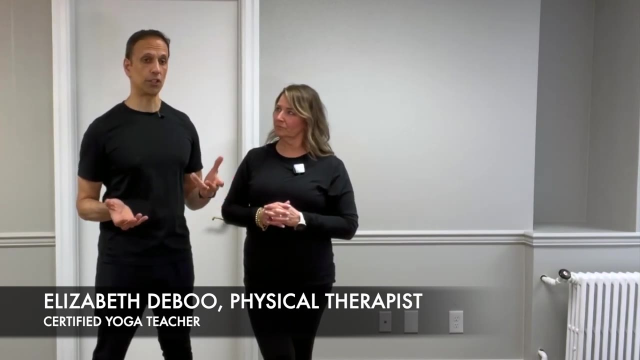 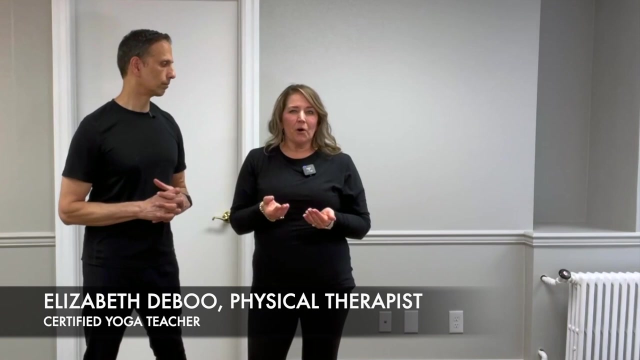 and continue to practice yoga just a little safer. In this video we're going to talk about specific yoga movements that we think we should probably avoid and then, where possible, can you show us some modifications, maybe for the exercise? Yes, I will try to do that. Some of these positions are just going to be a no, especially depending on. 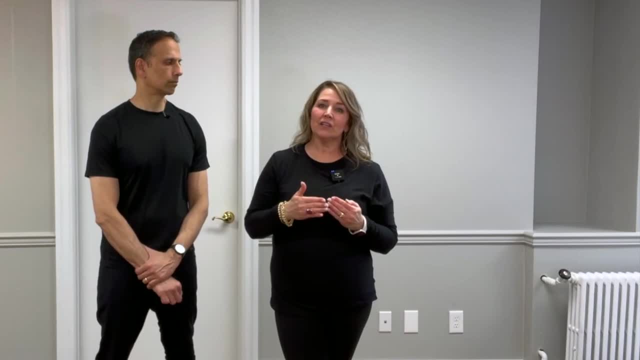 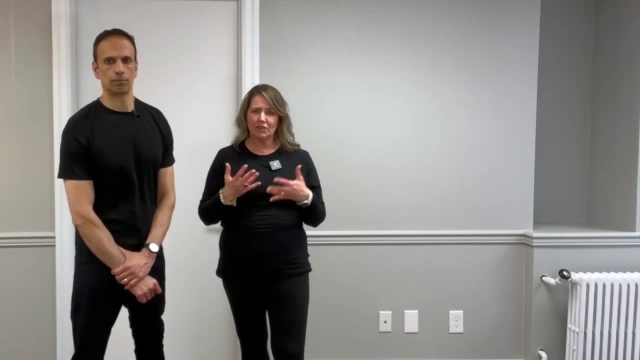 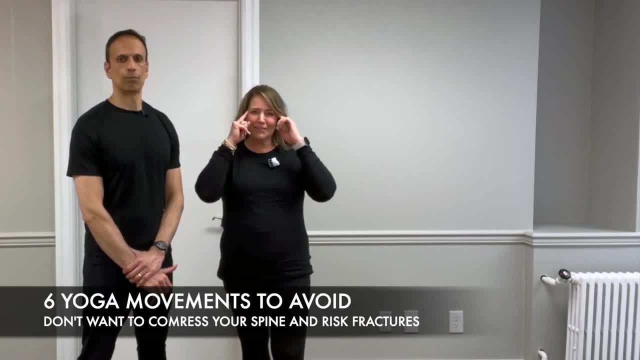 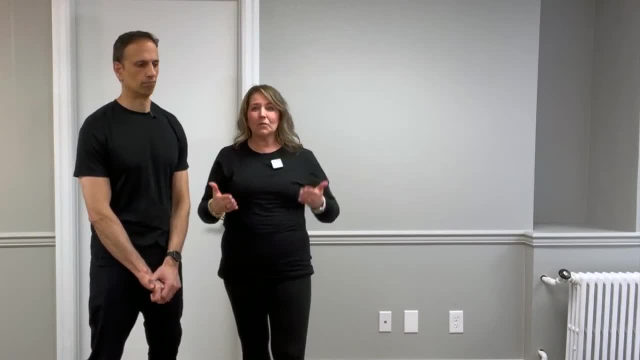 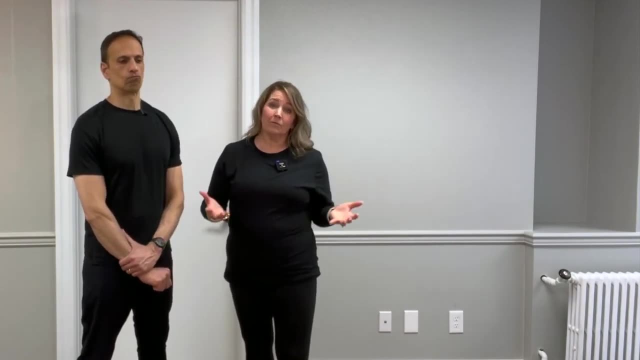 six things that you're going to avoid and then try to just like conceptualize this and transfer this over to other postures, because most yoga classes have in a series. they'll have forward folds, and we really want to avoid forward folds. Now the one that I want to talk about today. 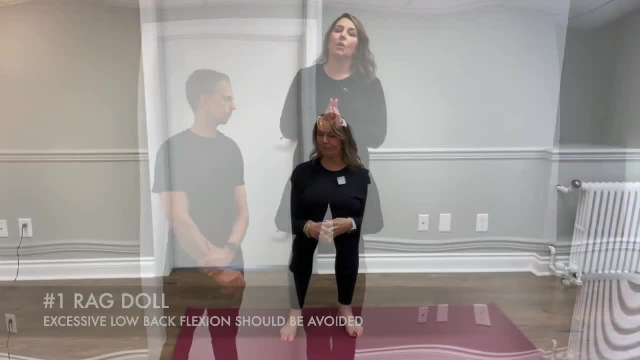 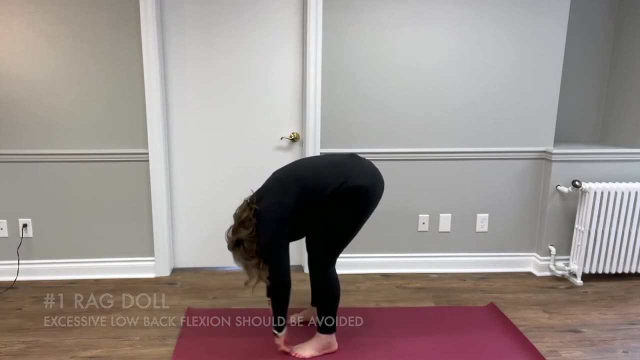 the forward fold is called ragdoll. So ragdoll, a really, really common forward fold- This is how ragdoll looks. Ragdoll looks like this And they're usually saying: dangle your hands and just let your body flow back and forth. Okay, This is one example of where you would see ragdoll. Oftentimes it's used. 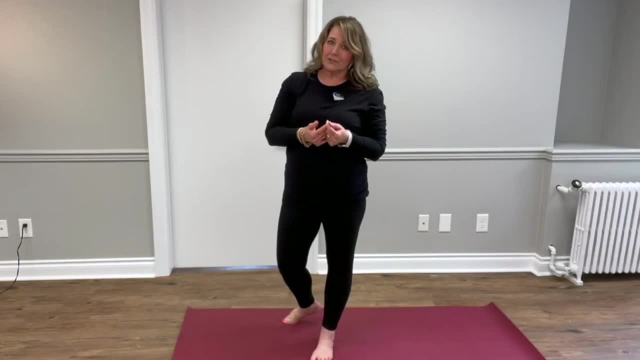 as a first part of the standing series. If you are challenged with osteoporosis, you really do want to avoid that. That's just a pure forward flexion that we don't want you to be doing. Okay, Instead, when the teacher is having people hang out there, you can just be in. 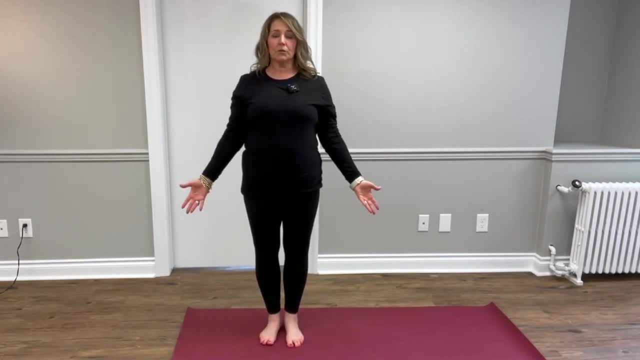 standing. You could do just mountain pose and really just take that moment to breathe and to center yourself and to feel your feet side to side. just really slow everything down and imagine letting go and follow her cues Only just transfer it into mountain pose If you want to further that. 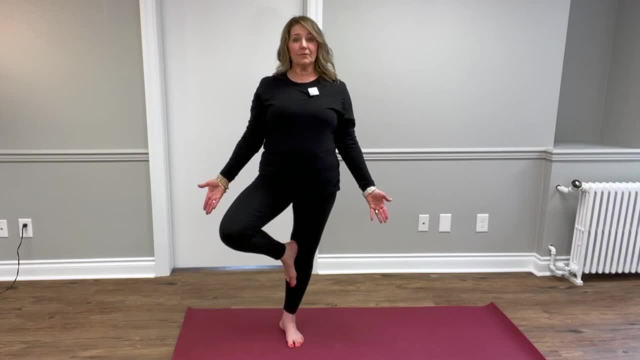 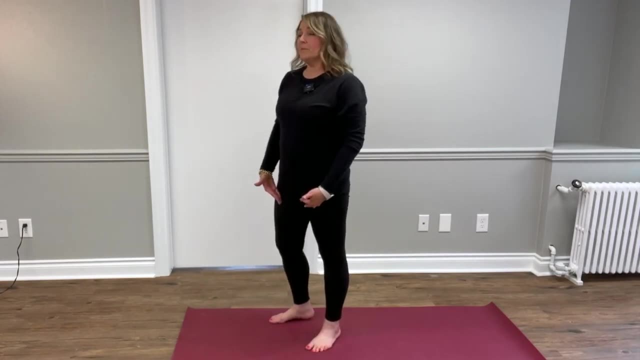 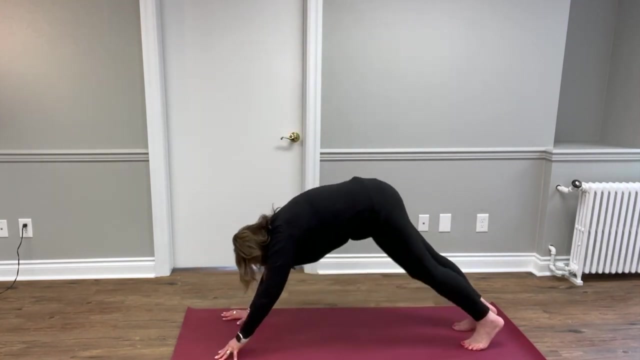 you might take it up into tree pose and just give yourself a little balance challenge. Okay, If you're in the middle of a flow class and you're doing sun salutations, So sun salutations look something like this. Let's say, you start in down, dog, and then you could flow up here. 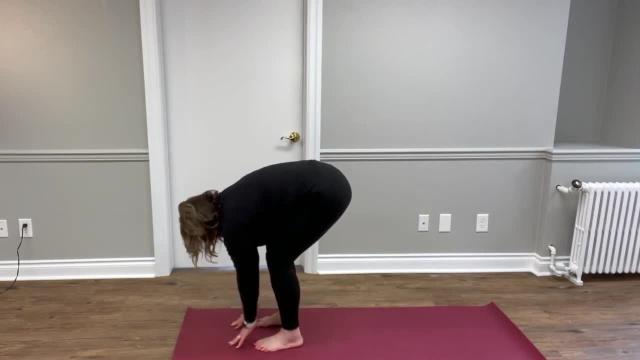 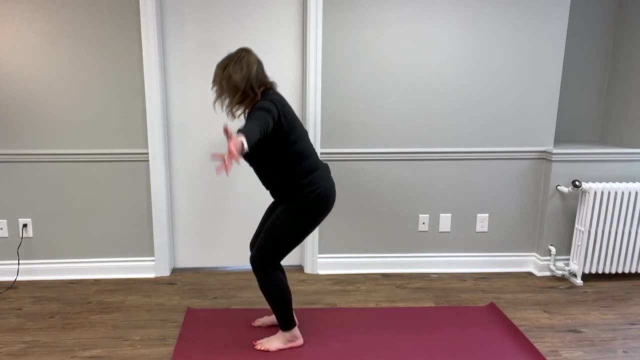 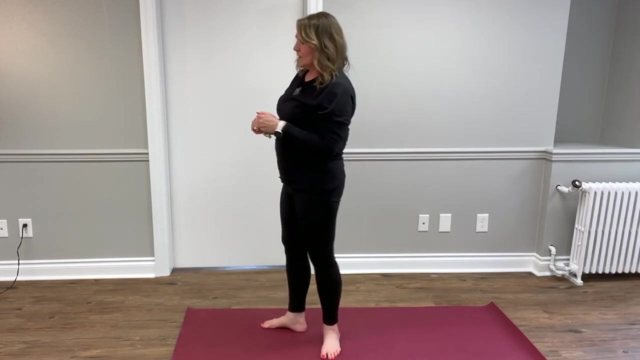 You usually start here in a forward fold. You come up here and then you go back to your forward fold. Then you engage your legs and you come on up. So you can see there was a couple ragdoll forward folds in there and you really want to avoid that. So instead of doing that whole flow, 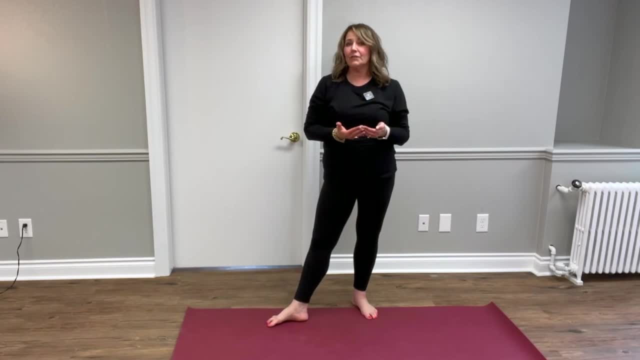 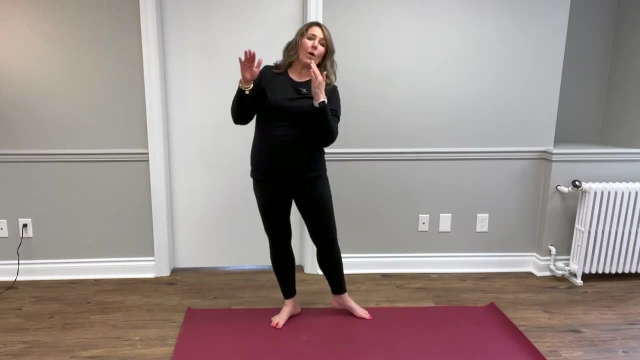 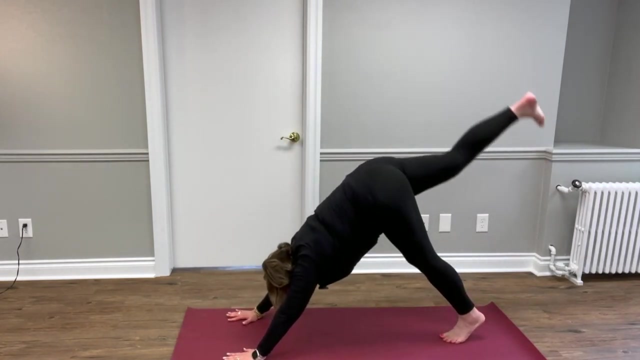 you might consider doing a different kind of yoga class. Do a hatha yoga class or a yin yoga class? Poses are more isolated as opposed to flowing one into the next, Because even going from down dog to we're still extending. we're still okay here, but I've got to get my foot through. 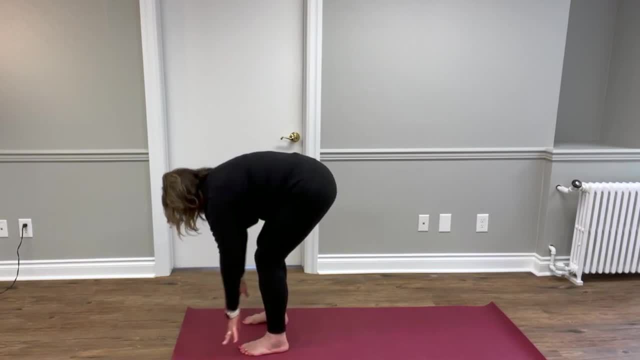 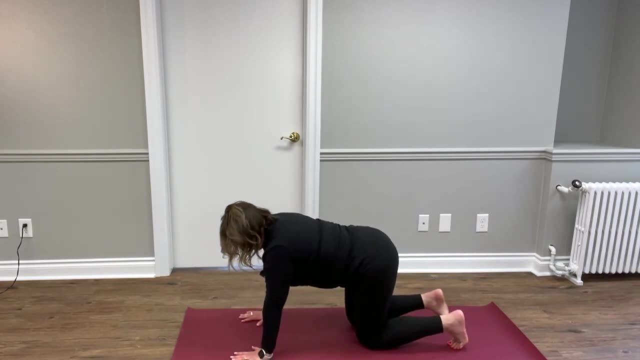 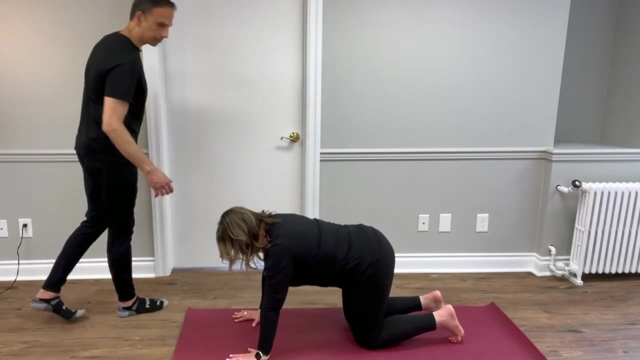 and then I'm really flexed already. Now, if you're right in the middle, maybe you'll go like this down dog, you'll come down to tabletop, but you still have to make your way up to standing pose, And so if you're down here on all hands and knees, what you could do is go into a half kneeling. 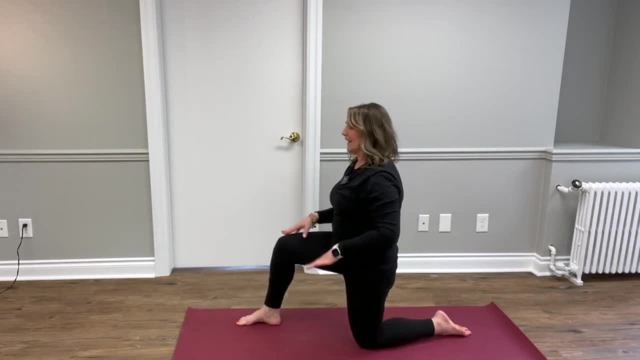 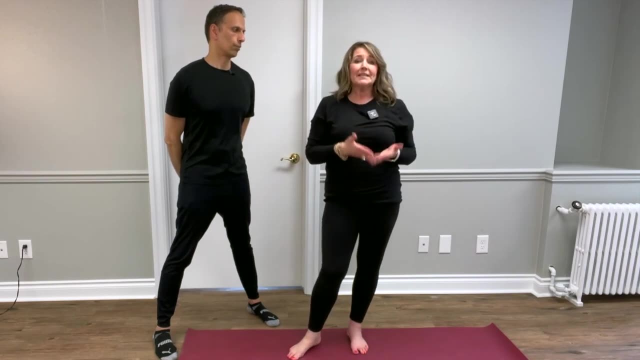 and then go to- or sorry, tall kneeling, to half kneeling and then just stand up from there, And that would be the safest way for osteoporosis. This is way we would talk to our patients. We would, we would teach them to get off the floor. 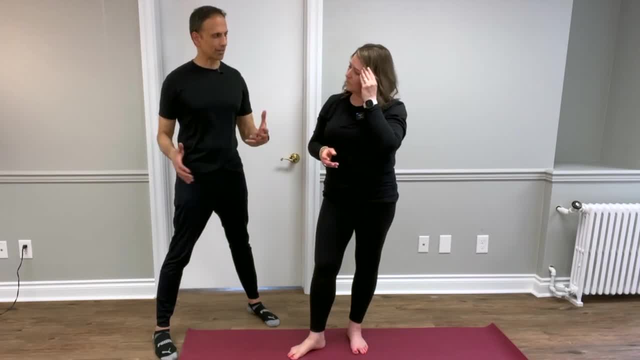 Correct. Yeah, Because part of it. the issue is too- is transitioning in and out of the pose, So like if somebody wanted to just get down on the floor to do a yoga series. sometimes it's challenging to work to get onto the floor. A lot of people will just do this. 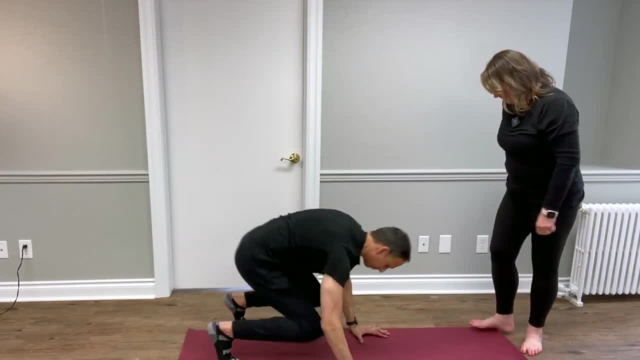 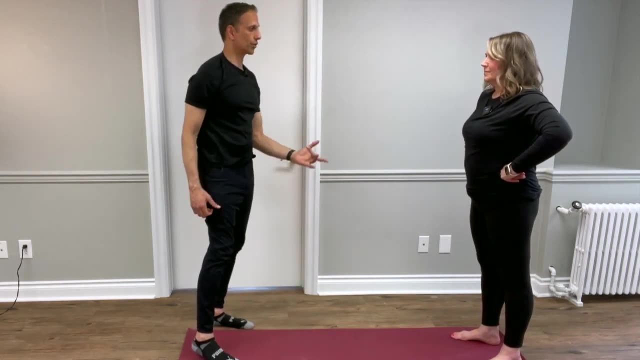 and let themselves down, But once again we've got all this flexion of our thoracic spine or lumbar spine that we don't want. And so just to kind of echo what you just said- how do we do this? were talking about. oftentimes I'll have people put their strong leg forward use. 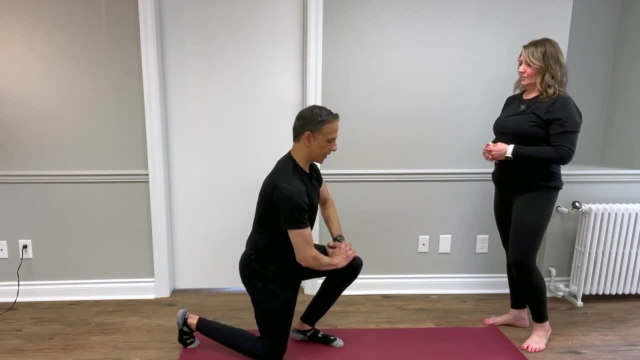 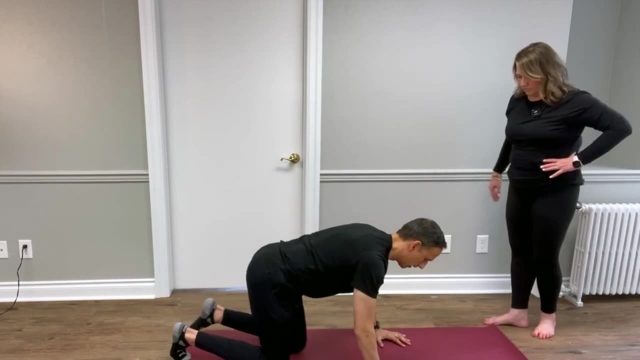 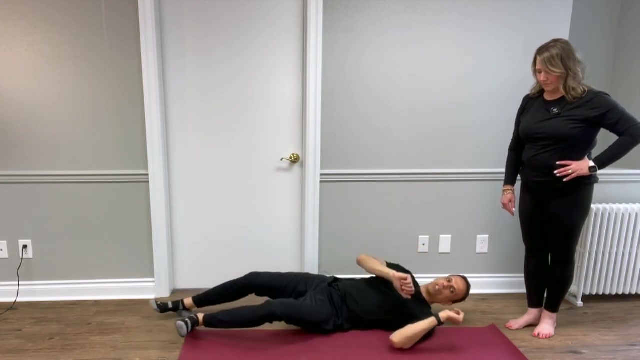 a supported hand if they need to, and come down to here, keeping your back still nice and straight. kick this leg back, come down onto your hands here and then you can side, sit and then do whatever you would need to do, and then, when you want to come back up, you would roll onto your side. first, come up to 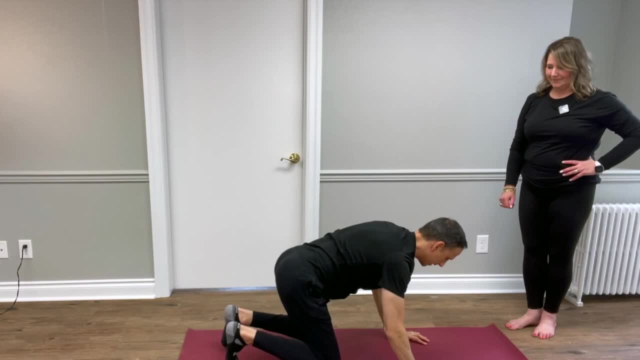 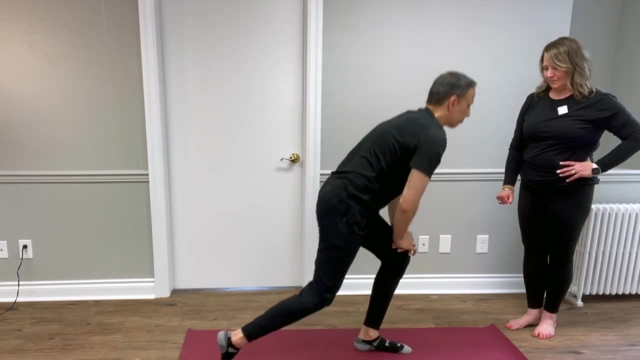 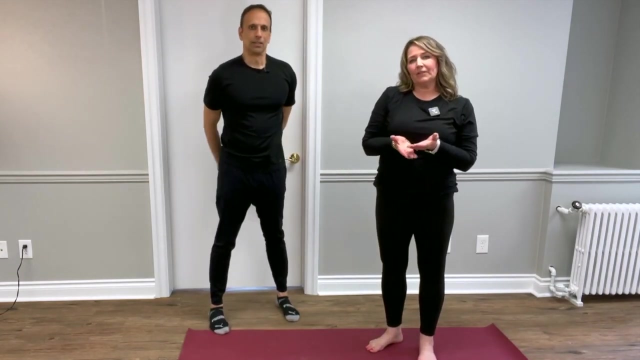 here, hands and knees, whichever your strong leg is, come forward, use your hands if you need to, or a chair for support, and then you would push yourself up again. yeah, so of course you might have to modify your class too. yes, and this is why I'm I'm giving you an idea to maybe take a hatha class, you might. 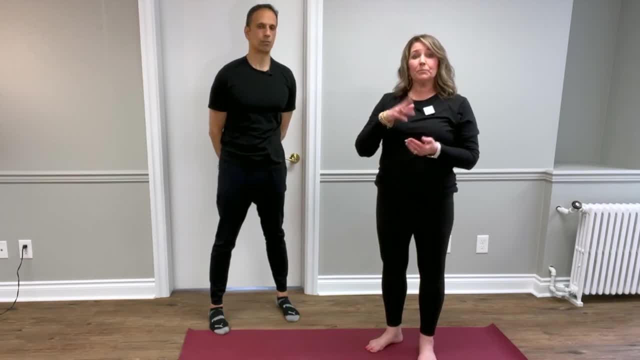 see a class that is described as hatha, as opposed to a power flow or a vinyasa. those are very flow classes that have a faster pace. that doesn't. they don't give you a lot of time to adjust in between each pose. you can still do the poses, but just isolate them so that you 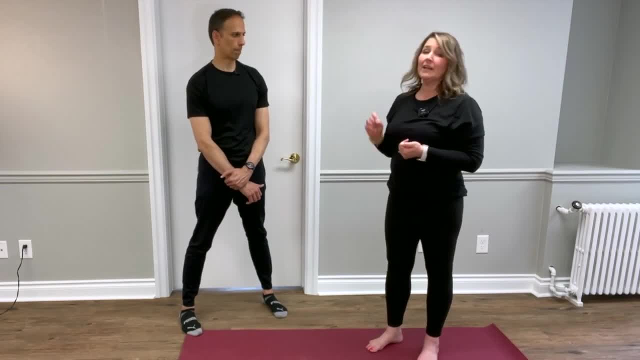 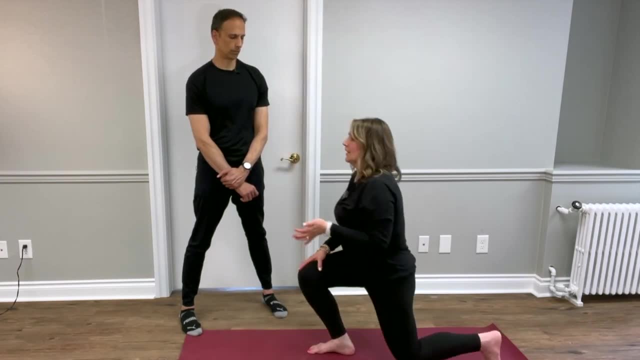 can customize. in a hatha class you would have plenty of time to do this transfer of you know kind of slowly, especially if you're doing this at home, going down onto one knee down here and down here. there's plenty of time to do that in a 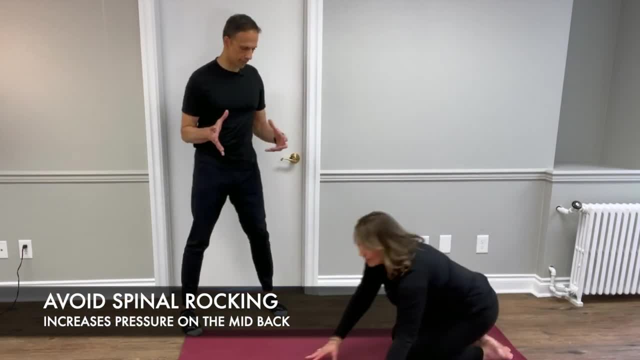 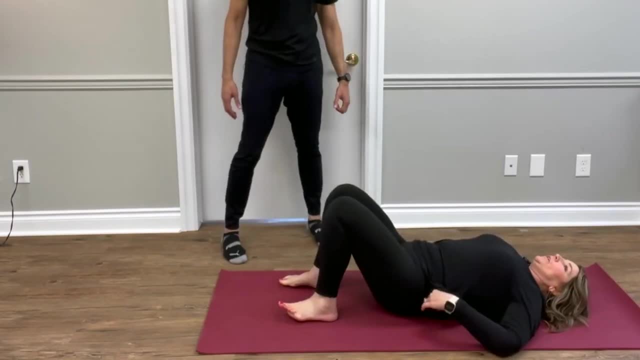 hatha class. now, what about spinal rockings? like I've seen? I've taken some yoga and I've seen some spinal rocking. yes, so what he's talking about with spinal rocking is, let's say we're here and we've done something, and the teacher says, go ahead. and they won't always say: 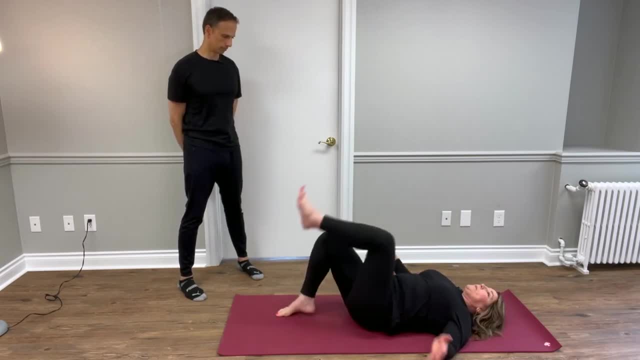 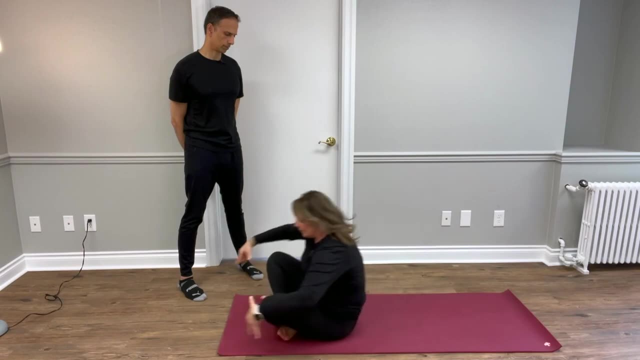 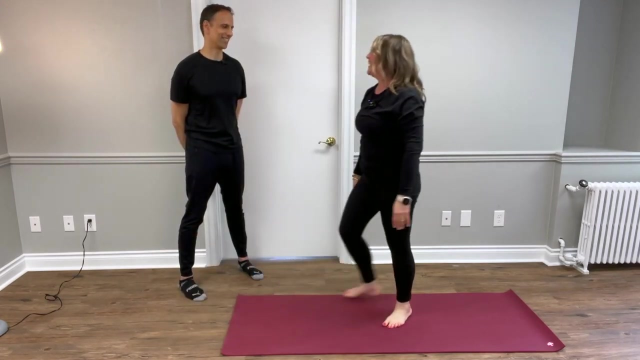 you have to rock yourself up, but they'll give that as an example, and spinal rocking is like this, and sometimes they want to do that to engage your core and then they want you to come up like this. some teachers end up like that- not me, I, but that's what they're talking about with spinal rocking- but you can see that. 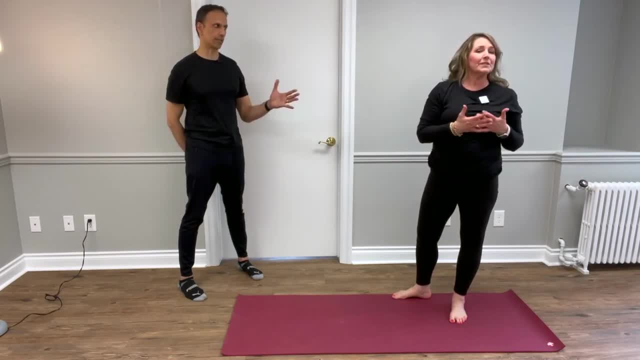 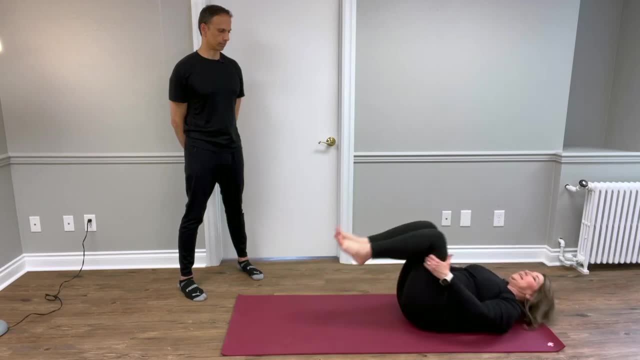 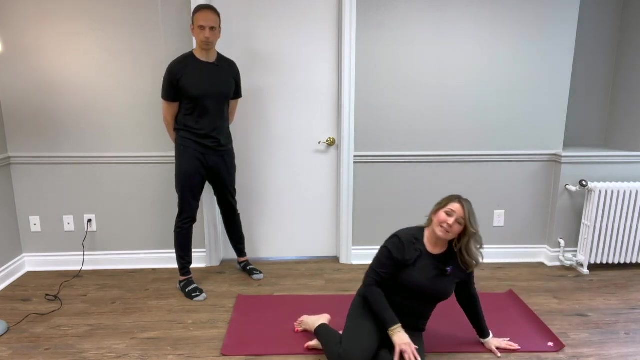 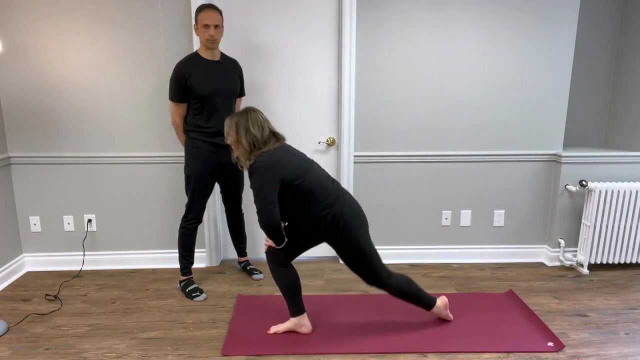 that's full flexion. so they probably want to avoid spinal rocking, definitely want to avoid spinal rocking. instead, you want to. instead of spinal rocking, you're just gonna come to your side, keep your spine as much in neutral, get up onto your knees and then strong leg press into your knee and come on up. 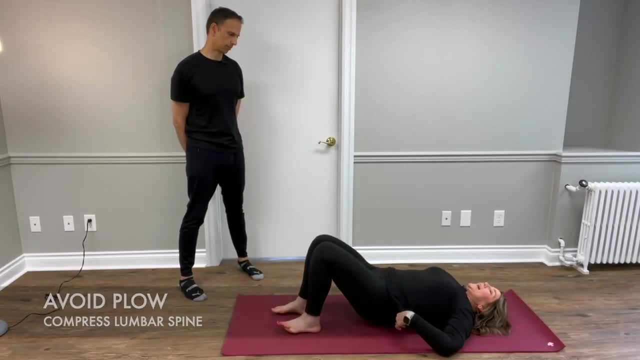 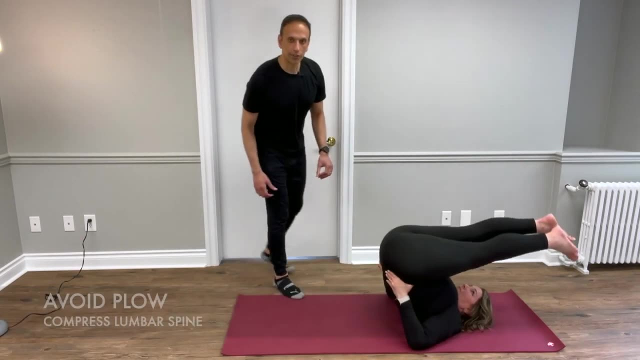 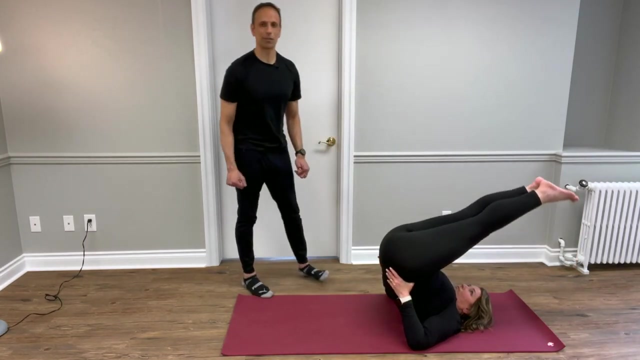 so now plow is another full flexion. I don't do a very pretty plow, but we don't want you to anyway. look at the amount of flexion she has, or thoracic spine and cervical spine, and so I get really nervous when I see anybody doing plow. 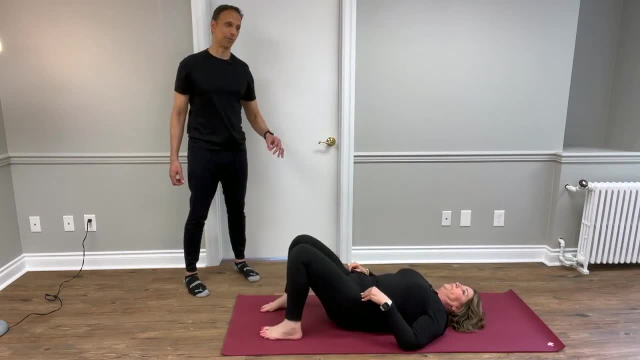 that doesn't even have, not necessarily osteoporosis or any type of spinal issue. I just get really nervous because the pressure it puts on that thoracic spine- yeah, it doesn't. it's a lot of pressure here, It's a lot of pressure through the ribs. 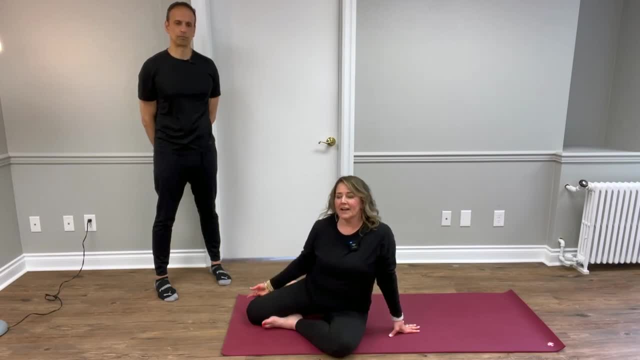 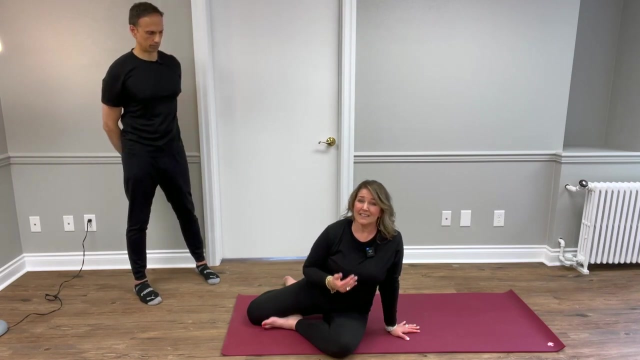 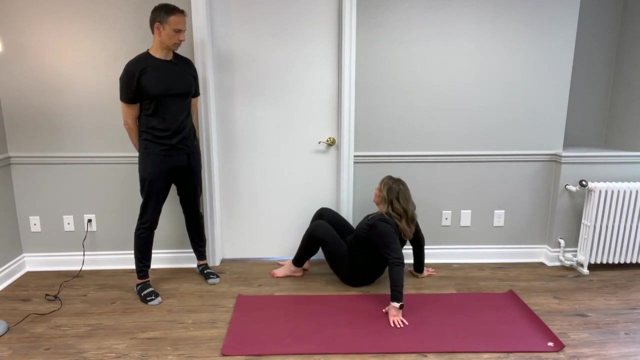 So, instead of plow, plow is really getting your feet above your head and they're actually folded over your head. So one of my favorite inversions- it's still an inversion and it's a safe, lovely, relaxing inversion- is legs up the wall. 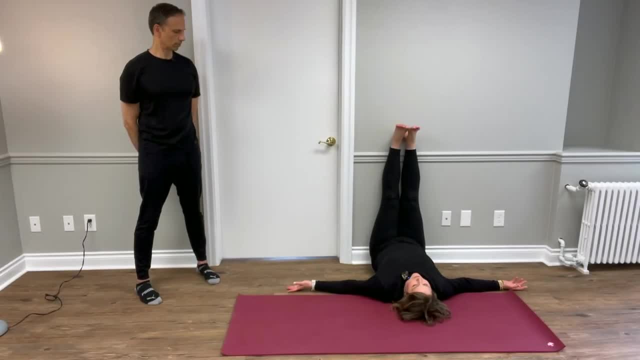 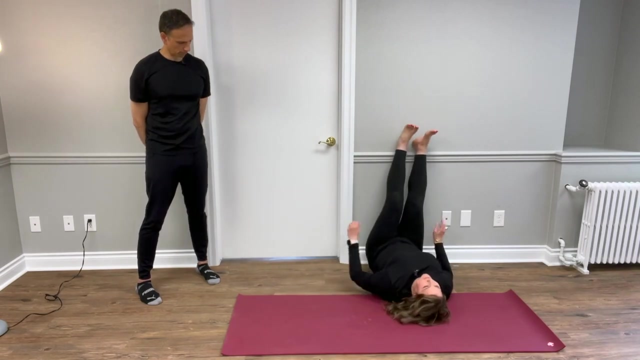 I do this a lot in my class and you just can be here And it's pretty straightforward to get here with a neutral spine and to get out, Come down, roll to your side and then come on up and then reverse. You just wanna make sure your bottom is pretty close. 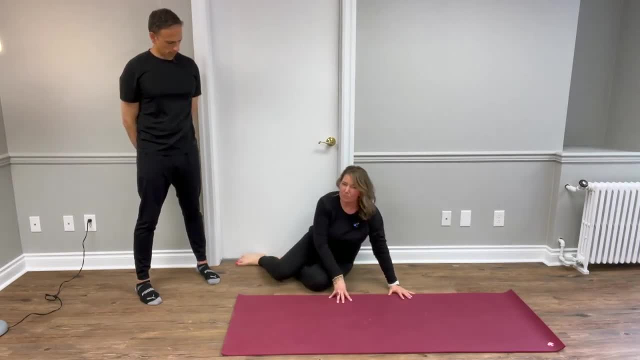 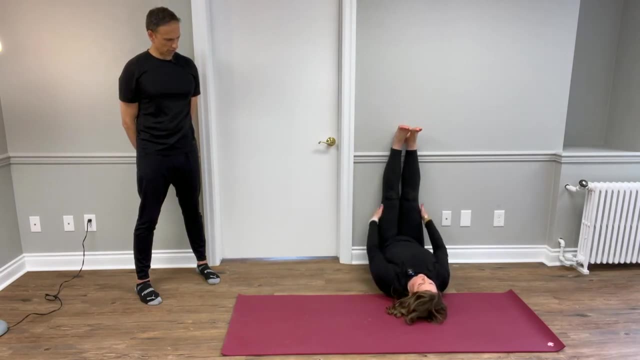 to the wall from the beginning. So get your bottom touching the wall and then you'll go to your side and then you'll just go up. Your bottom should be touching the wall and then you're fully supported And then you have your nice. 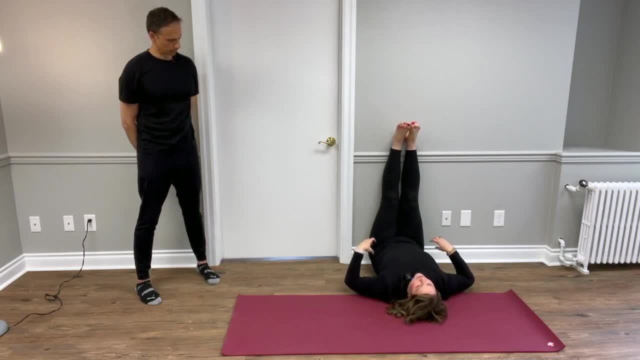 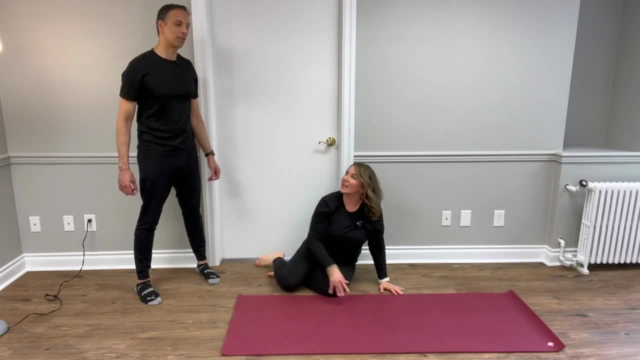 good inversion where you get that relaxation. The blood's draining from your legs and it's just amazing. That's a much better alternative than the plow- Much better. it's more comfortable And I just think it's easier to get into. it's safer. 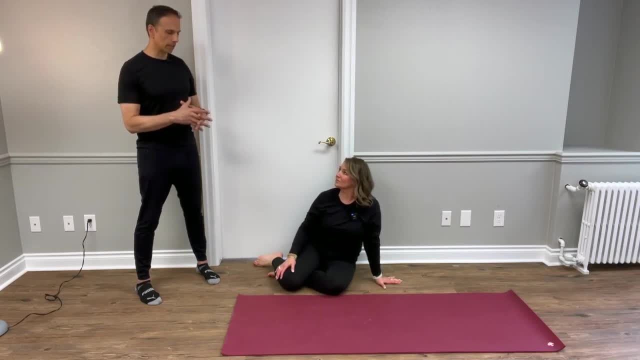 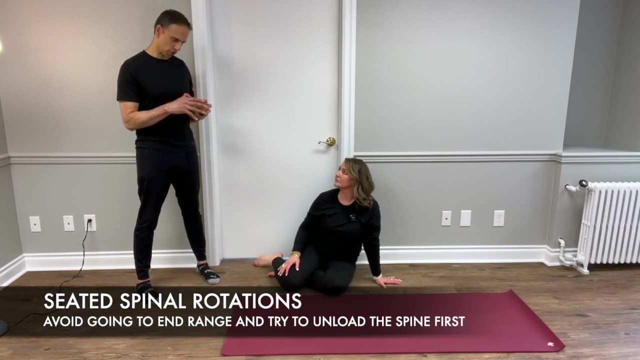 Now, what about a seated like? let's say you're in a class, whether it's yoga, Pilates, what have you? and they're doing a seated rotation? I get a little nervous. I get a little nervous, Yeah. 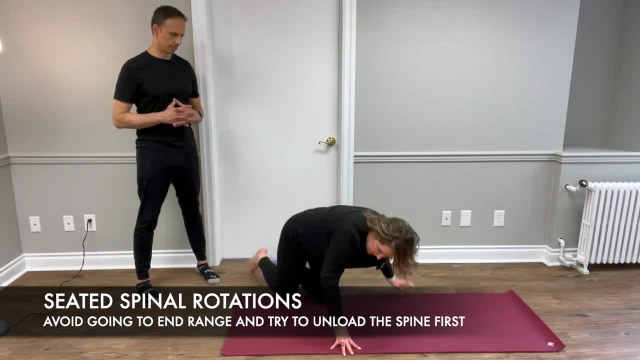 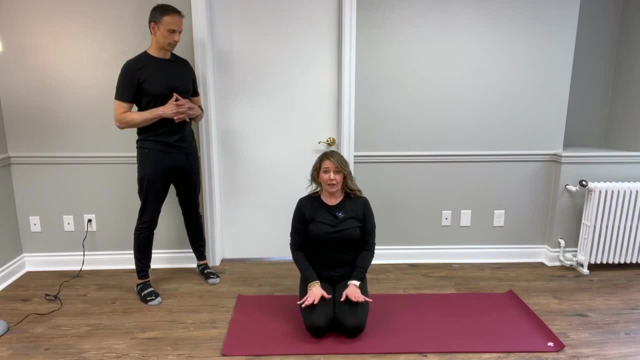 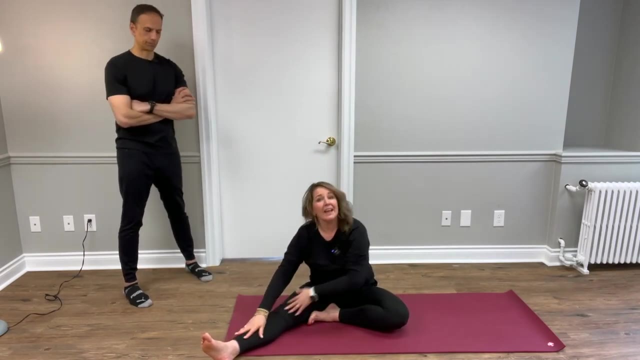 Because of the loading of the spine. So by a seated rotation it means really anything that is like this: Yeah, Like this, right, And so you wanna avoid any rotation. A lot of times you'll see this in yoga class, where they want you to rotate right. 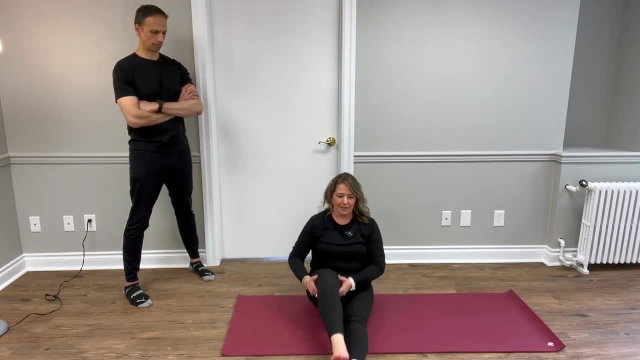 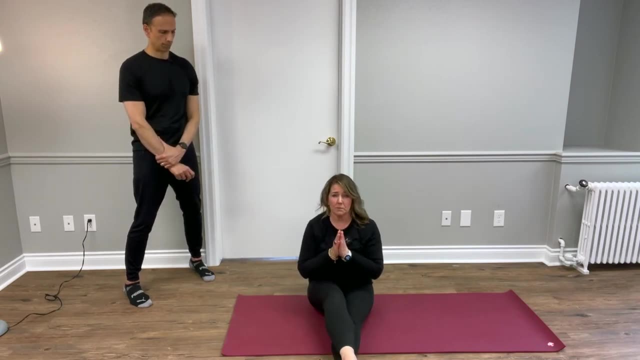 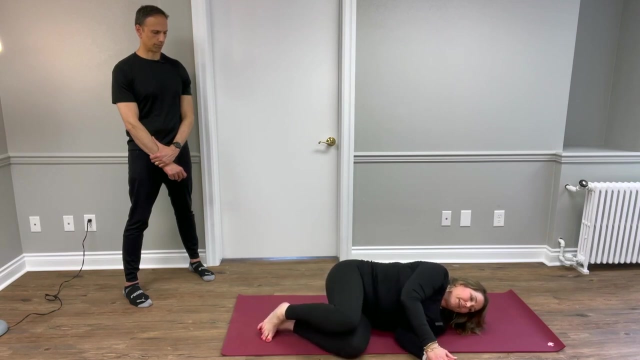 That's a seated rotation. Another seated rotation is this: When you're doing twists or rotations, we want your spine to be unloaded, And what that means is that you're going to be on your back or in sideline. And my very favorite rotation to show people is this: 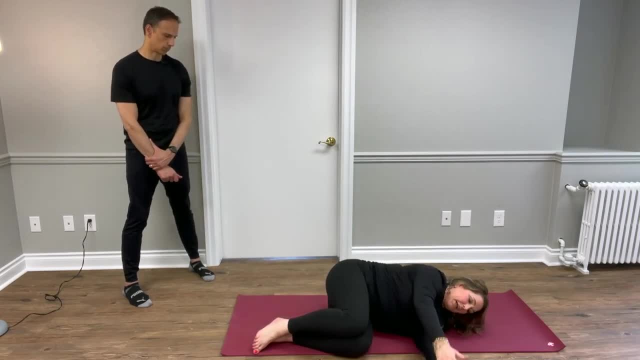 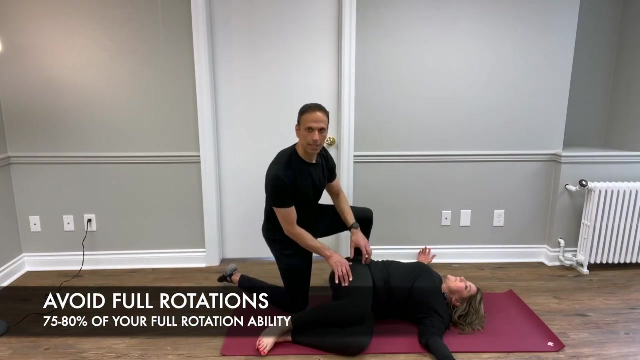 It feels really, really good. You're in sideline, your spine is unloaded, You can put a pillow underneath the back arm, So if you feel like a strain anywhere along your spine, you can bring that arm up and support it. One thing to remember, too, when you're down here, is that 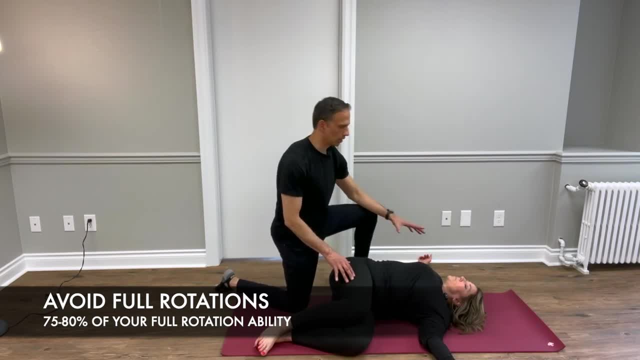 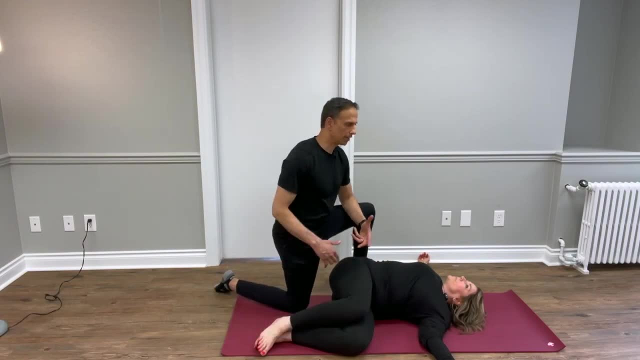 you don't wanna force that rotation. You might wanna go maybe to about 75, 80%, but not necessarily, definitely don't ever wanna push it down. I mean living life without rotating, especially when you're standing and sitting and rotating. 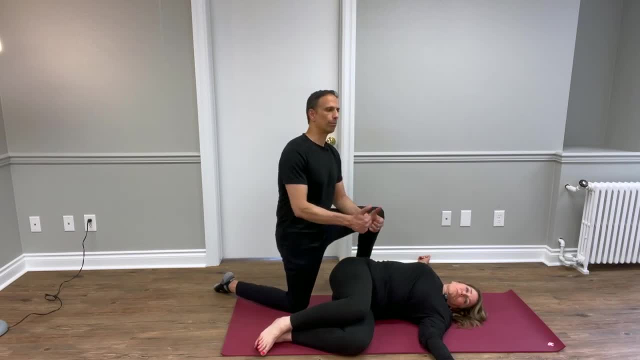 isn't really functional. But what we're talking about is the repeated rotation that we might do in class, Because if, from a functional standpoint, I might not just sit there and rotate over 10 times to one direction, That's not very functional. 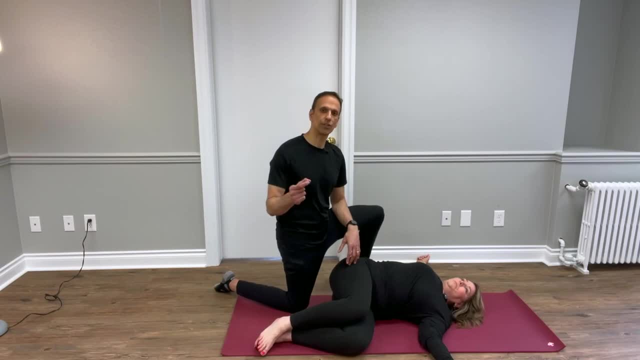 but I might do something like that. if I'm in a stretch stretch class And that's when you need to say, okay, you know what, I shouldn't probably be doing- so many seated, repeated flexion twist exercises- And that's when you wanna come down here and lie down. 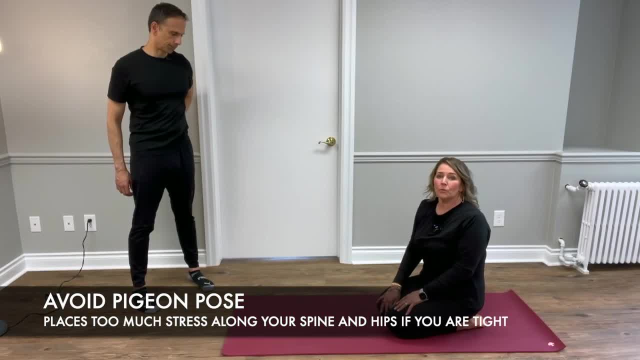 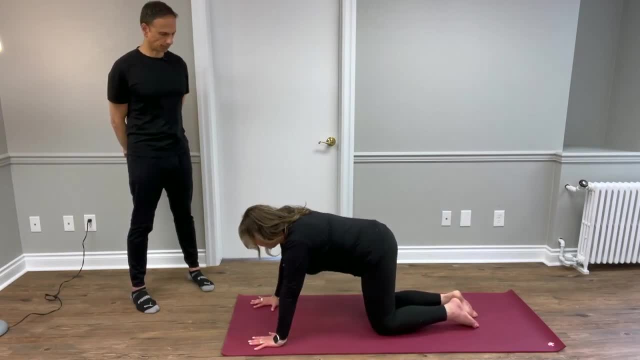 and do something that's unweighted. Okay, the next posture we'd like you to avoid is something called pigeon, And this is where I'm gonna just show you like you're still okay here, but you have to really flex your spine to get your leg up. 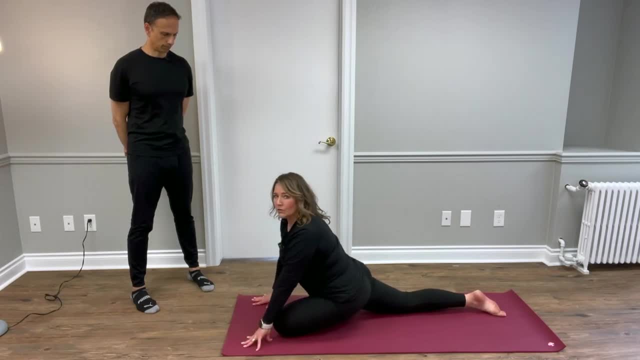 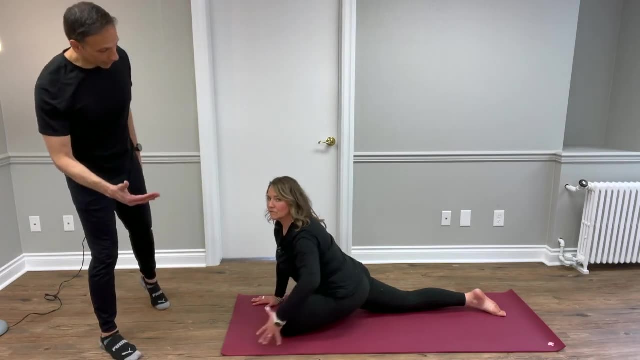 and to attain pigeon. okay, Once you're here, you're actually okay. Your spine is actually an extension. Yeah, it is putting some compression through the hip, But yeah, definitely compression through here And if a lot of people are tight. 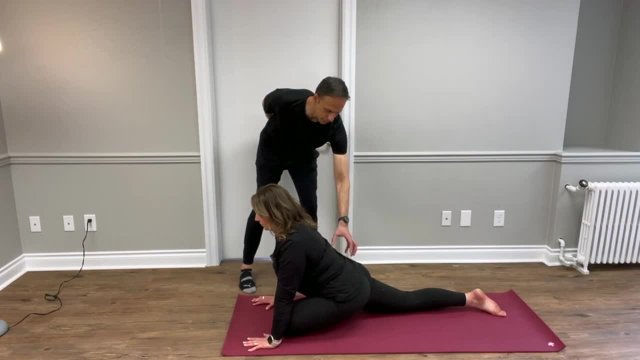 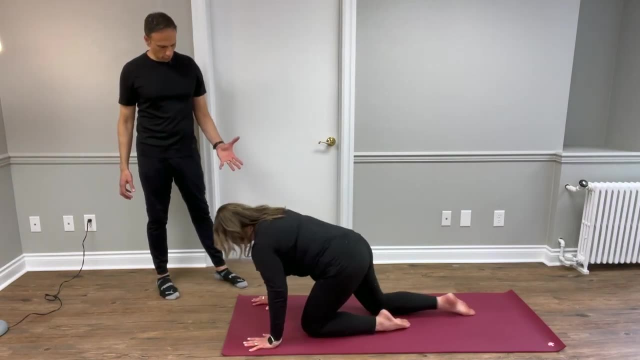 they can't get this neutral spine and they end up getting a lot of flexion not only from the lumbar spine but from the thoracics, And I guess this is where something Elizabeth like would a one-on-one help, Like if someone isn't sure. 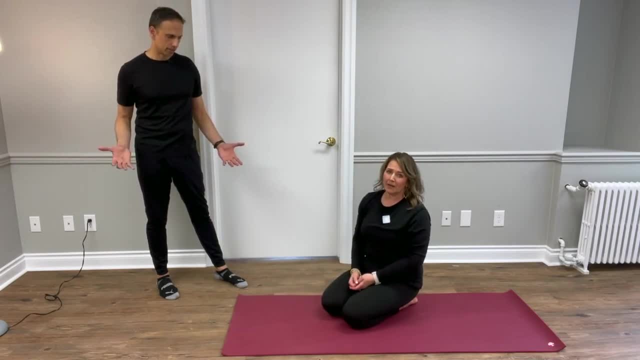 because everyone's coming in a different place. Yeah, I would definitely recommend a one-on-one, because even these that we're gonna say here in your mind, you're gonna be going. oh well, that reminds me a lot of this. 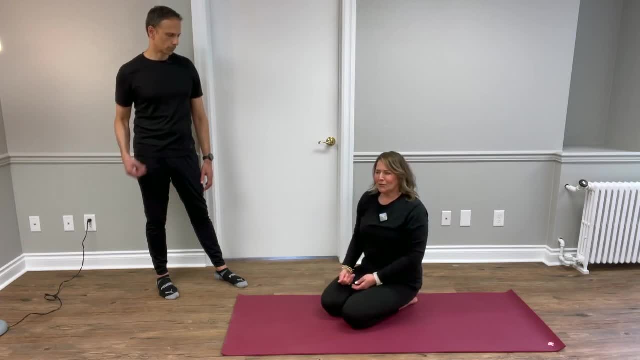 And that reminds me a lot of this. And then you're gonna get into your yoga class and it's gonna be a little bit stressful And you're gonna be like this is really counterproductive to what I wanna get out of yoga, And so I think, yes, a one-on-one. 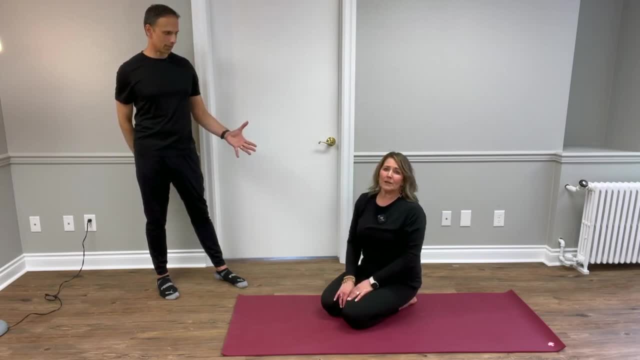 So they can even do one-on-ones with you. Yes, you could do one-on-ones with me or anybody local to you. Well, we can do it on Zoom. Oh, we could easily do it on Zoom. So reach out to us and Elizabeth will be able to do that. 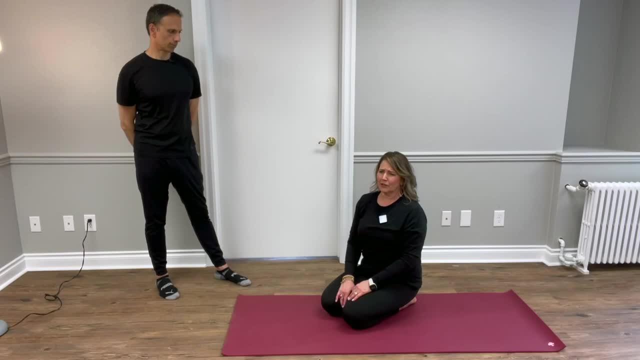 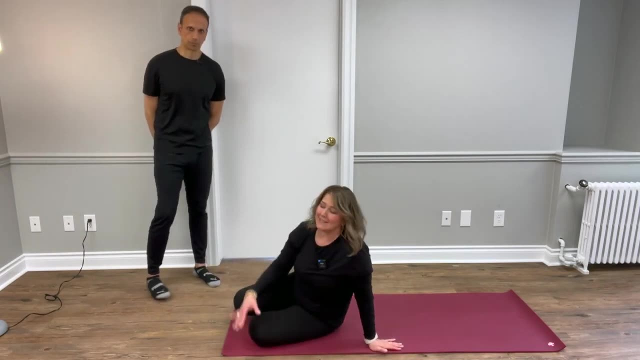 for you on Zoom. Absolutely. I'd be really happy to do that if you'd like to do it on Zoom. So now, instead of pigeon- and a lot of people, even who don't have osteoporosis, take this as an alternative- You get down on your back. 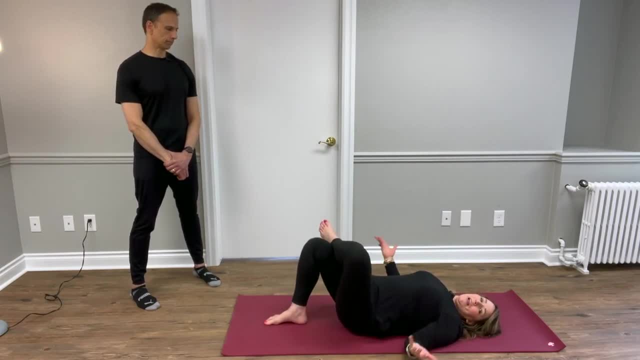 and you're gonna do a figure four- Same thing- but your back is unloaded and in neutral and it's just safe and lovely. And then you're just gonna reach through, And the thing you wanna remember about figure four is: you don't wanna be up here. 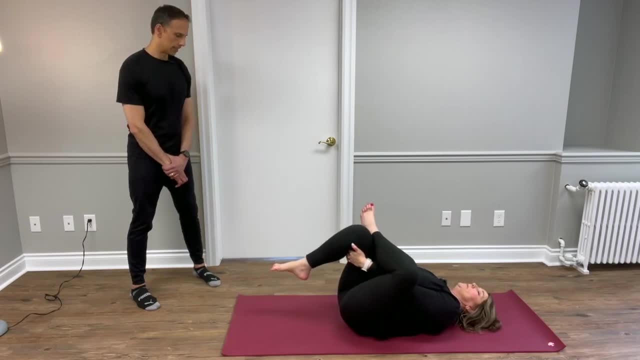 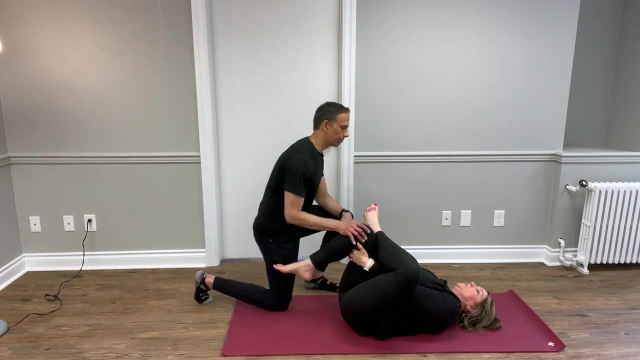 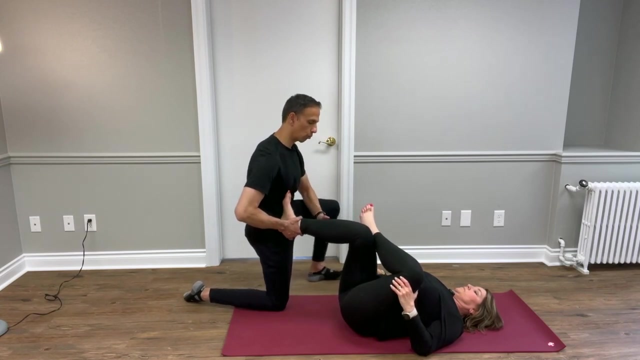 because you can see my spine is flexed here. You wanna be able to grab your legs and keep your spine and your head on the floor, And if you can't, you can get a towel or a band. Another modification would be is to do it up against a wall. 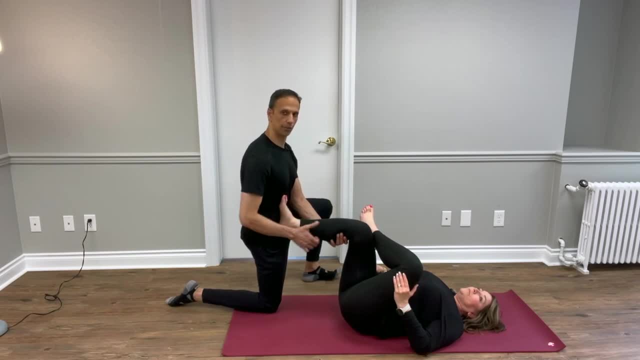 So pretend I'm the wall right here. That way you could come in a little closer to the wall if you want more of a stretch. but that way your back is nice and straight and you're getting a nice hip stretch, but without straining on the spine. 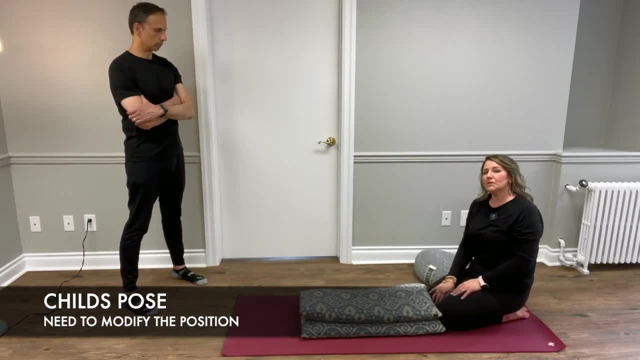 Child's pose is really, really common and it's almost it's so common. it's our reset pose a lot of times if you're feeling fatigued in a yoga class, or it might be the way you start in yoga class, or they suggest as a, you know, as your home base. 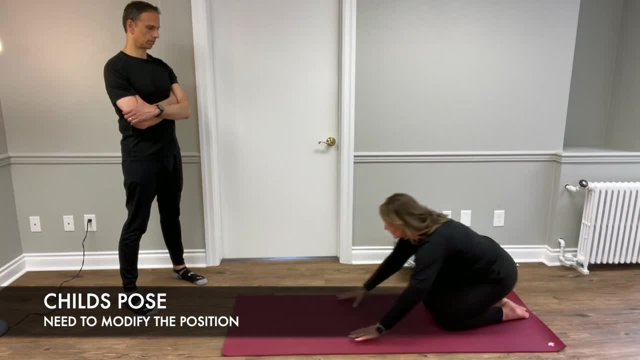 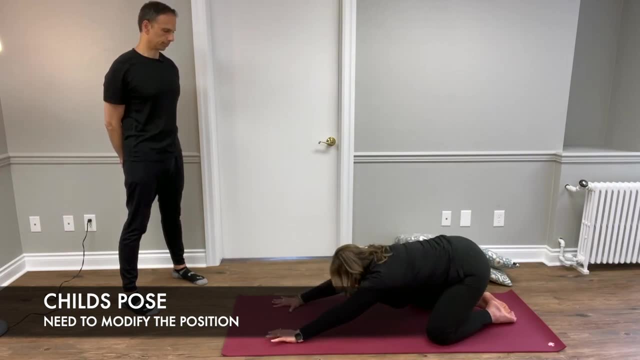 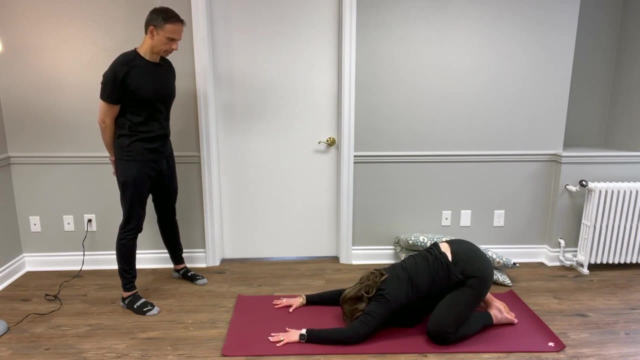 So child's pose- traditional child's pose- is like this, where your knees are apart, your toes are together, you're reaching your hand forward and you're coming back, head is down. So once you get here, you can be in neutral. 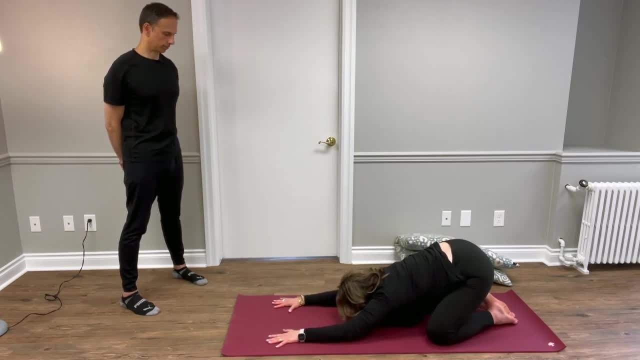 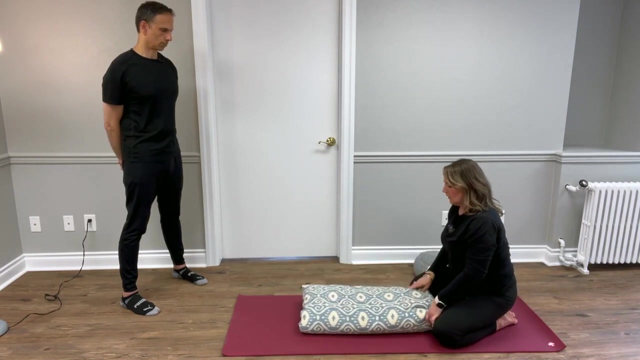 Some people don't have that much extension of their spine like this. Some people can't put their forehead on the ground, And so, instead of going through and wondering, am I in, am I in? flexion, What you can do is just keep yourself in neutral. 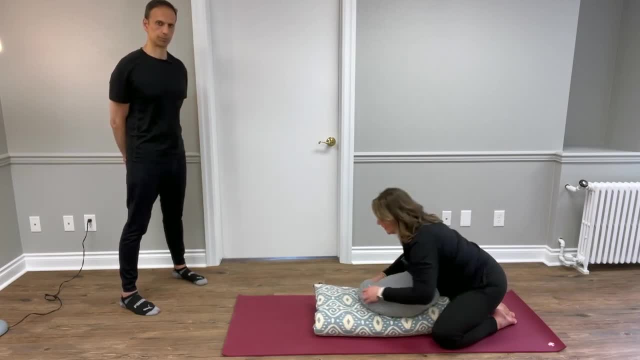 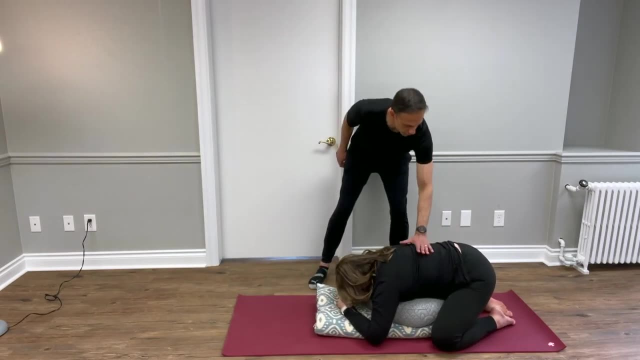 So that might take stacking up some cushions. So here we go. So keeping yourself in neutral here And what you're after is a nice flat back. Notice, she doesn't have that hyperkyphosis through her thoracic spine as well too. 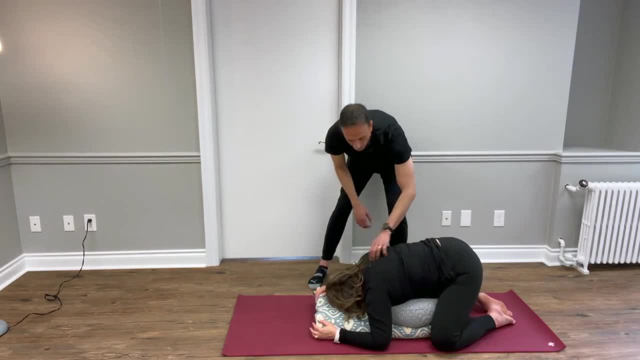 And if she didn't use her fist, go ahead and drop down for me. Do you see how she starts to get a little kyphotic through here? So then bring your fist back up again, And then she's just nice and flat. 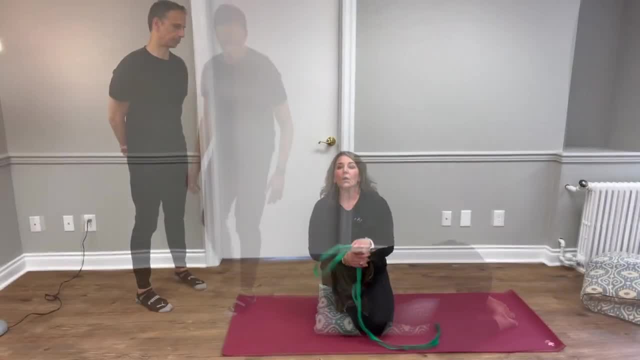 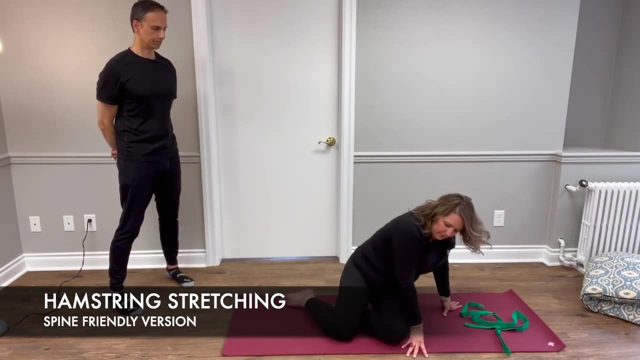 And then she's just nice and flat through here, which is just a great substitution. Okay now, another thing that we often do in yoga class is a hamstring stretch That might look like another. we in yoga it's usually a combined movement. 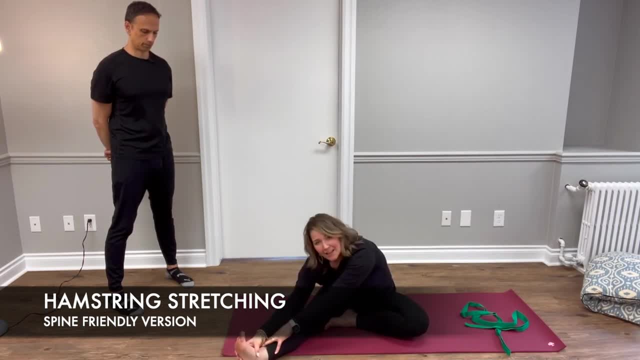 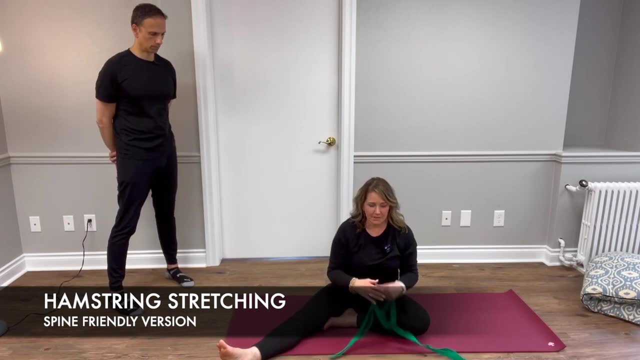 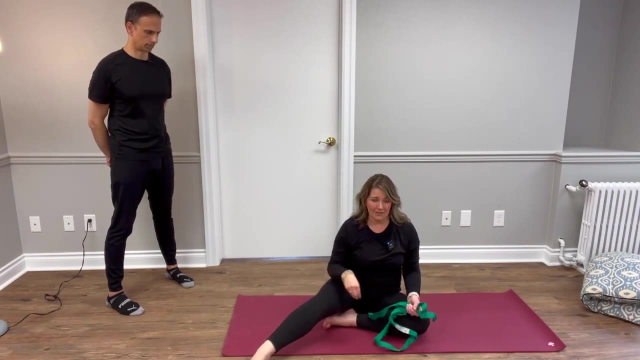 And so we have our spinal twist and hamstring stretch. So better in these cases for osteoporosis, we want to isolate those out. So we already talked about this. We already talked about the spinal twist. We want to do that on the side, on the back unloaded. 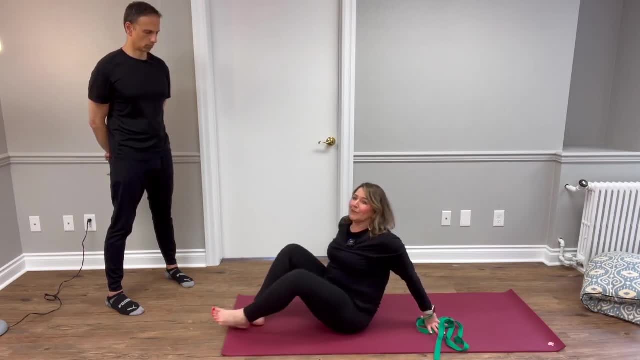 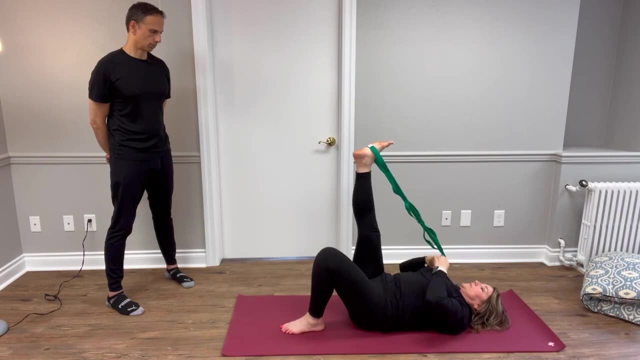 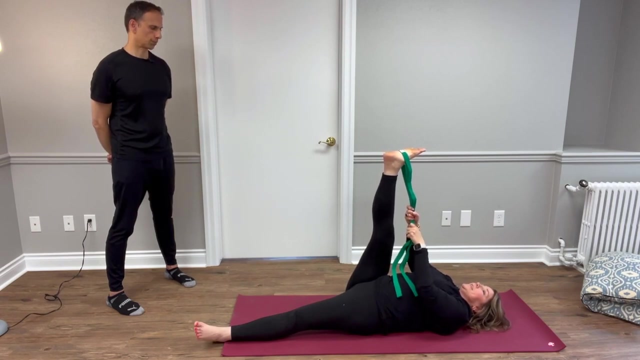 starting off in neutral And we talked about the figure four And when you're doing your figure four you could just take, you could take a strap and just do your hamstring stretch here and really let it be comfortable for your back. And so you're just thinking here about hamstring. 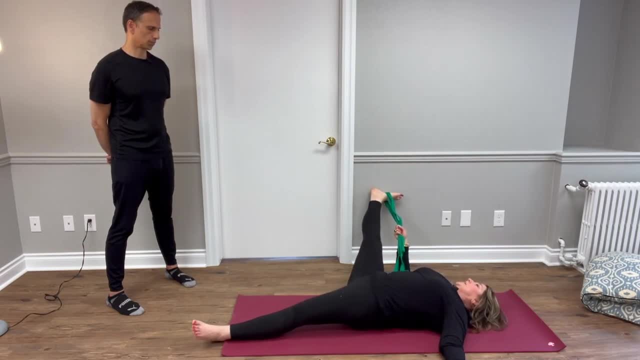 Now another thing you could do if you're next to a wall hamstring and you can get a little bit of the inner thigh stretch too. just make sure you have something to rest your foot on, And this is really really, really nice stretch for the hip. 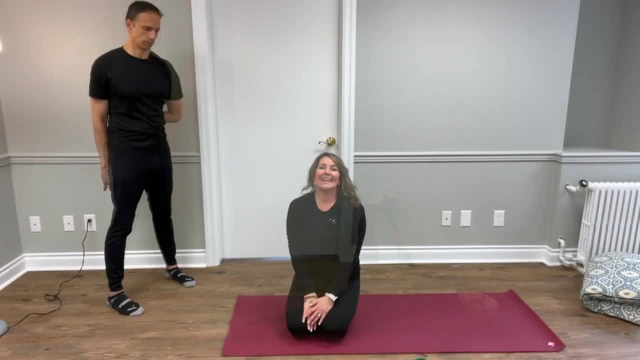 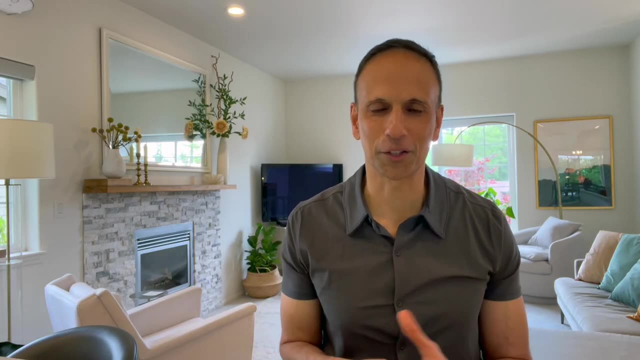 for the hamstring and for the inside of the thigh In the next video, the fun stuff, the yoga poses that we encourage you to do. All right, everyone. if you've made it to the very end of the video, congratulations. hopefully you learned something. 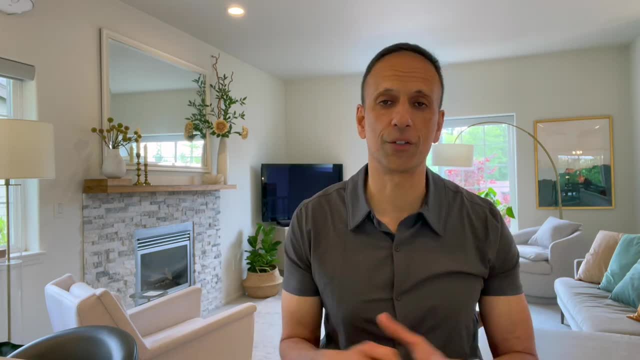 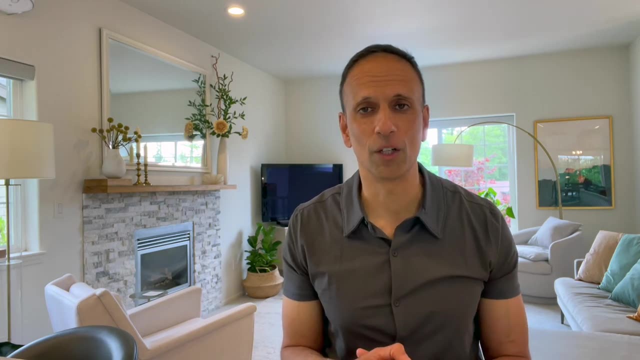 I remember you can work one-on-one with Elizabeth as well, too. if you ever want to Zoom or a tele session to kind of get dialed in on what you need to do, All right, if you haven't subscribed, please consider doing so.